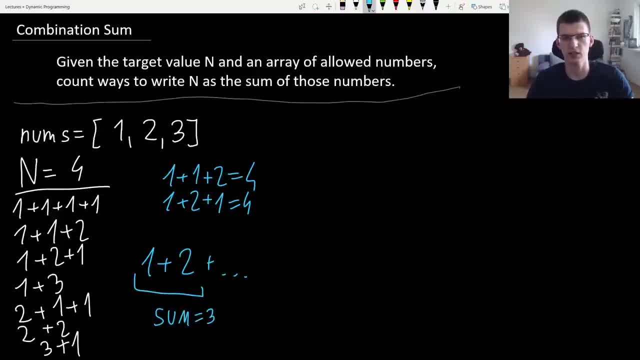 know the sum is 3 and this suggests that this should be dimension of DP, the state. Since we are counting the number of ways to write n as something, then DP will be int, DP of some dimension state, and that int denotes the number of ways. DP of i will be the number of ways. 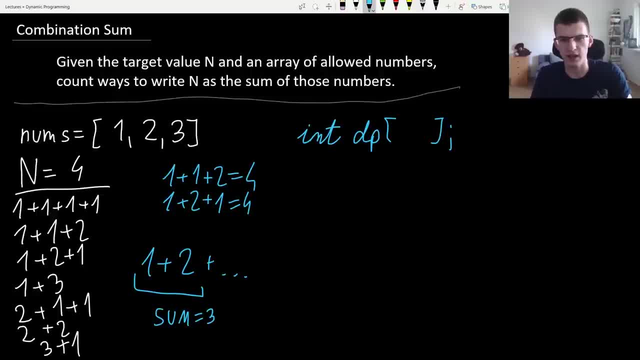 that we are at state i and i denotes the sum. i is the sum so far. Then we can in some way initialize that I will say DP of 0 is 1 and then what transitions we can make If we have sum equal to 10 and the allowed number. 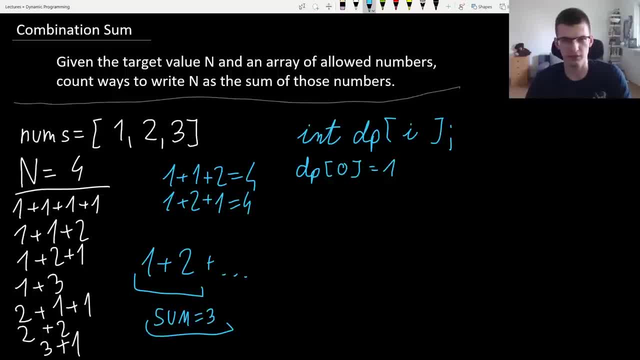 are 1, 2 and 3, then I can get sum 11, 12 or 13.. Let's see some implementation of that. The first code is quite standard. We initialize DP of 0 as 1.. There is one way to get the sum 0,. this is just empty sum, and then we compute every next DP of. 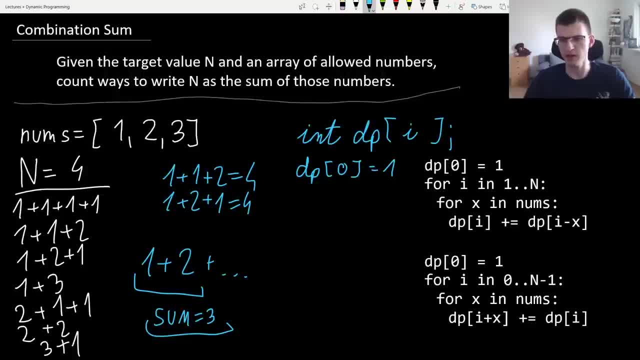 i. If we want to get the sum i, then we iterate over the last number, x. We can even simulate that with our example of 0 is initially 1, then every next one is 0 up to dp of 4 and every next one is computed. 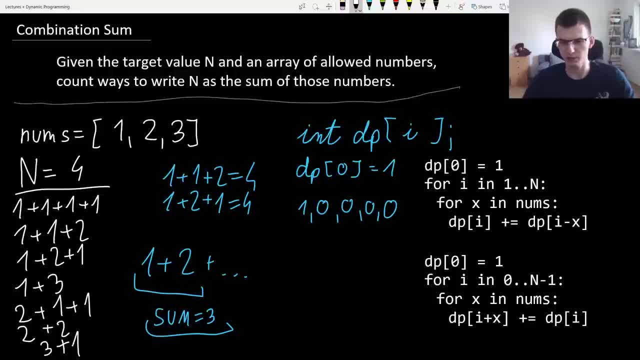 as the sum of three previous values, quite similarly to Fibonacci numbers, where this will be 1,, this will be the sum of dp of i-1 and i-2, which is 2,. this one will be 4, the sum of previous three numbers and this one will be 7.. 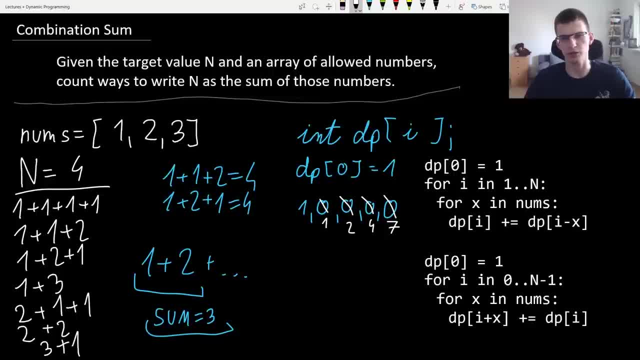 The second approach is a bit different. it's so-called forward or push dynamic programming, where we already know value dp of i and we use it to update future values. We again start from the array 1, 0, 0, 0, 0, then we start from i equal to 0 this time. 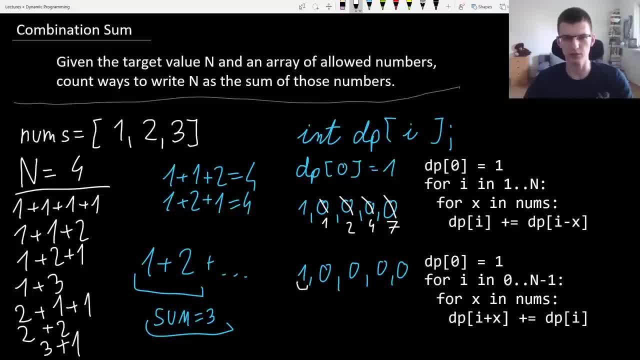 we use 1 to increase future values. we know that there is some number of ways to get the sum. We add sum equal to i and we consider next element to add to update future values For this one. we'll update this 0 to 1,, 0 to 1, 0 to 1, every next three values because 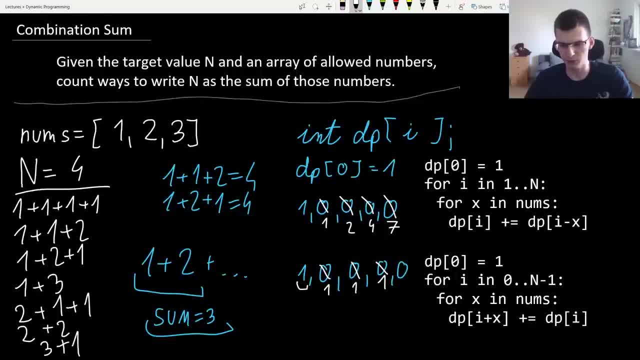 in our example nums are 1,, 2 and 3.. Then we are at this i, the value is again 1, we update next three values: 2,, 2 and 1.. We are at i equal to 2, we increase future values and finally, here, we increase dp of. 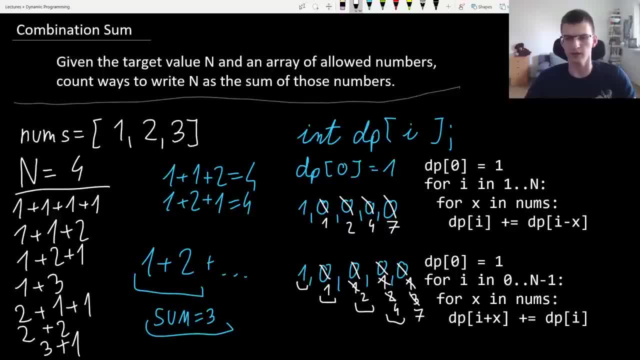 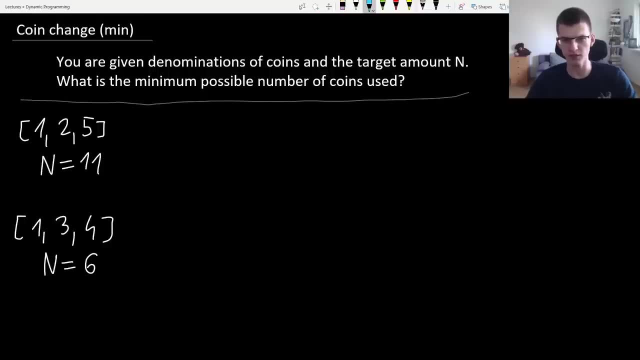 n by this value 7.. Computed values are the same, it's just that the method is different. In the next lecture we'll see more examples of this forward dp. The next problem, coin change, is quite similar. We are given denominations of coins and the target amount, n. what is the minimum possible? 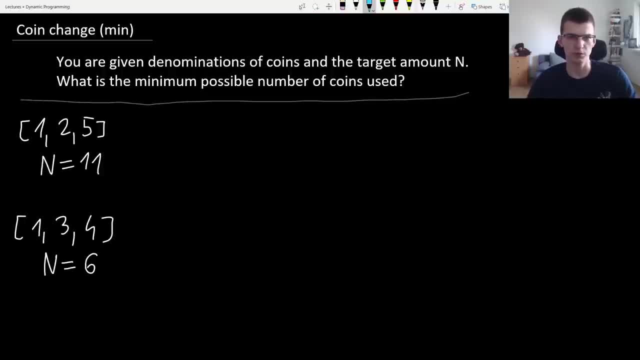 number of coins used. The main difference is we previously had to count ways and here we are finding the minimum possible number of coins For n equal to 11 and coins 1 to 5, I can get 5 plus 5 plus 1, this way I get the sum 11. 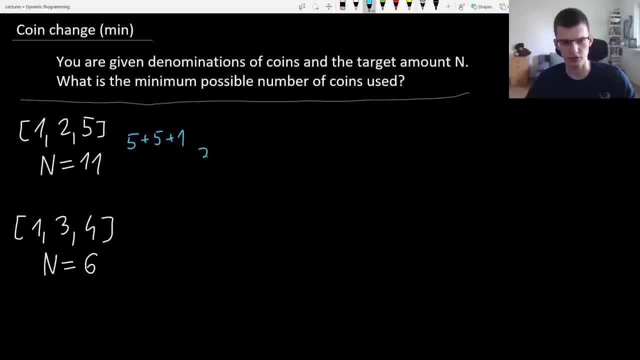 and I use 3 coins, so the answer is 3.. It's impossible to use fewer coins. In the next one, I can use 3 plus 3, 3 plus 3.. It's impossible to use fewer coins, so the answer is 3, 3 plus 3,, 3 plus 3, 3 plus 3,. 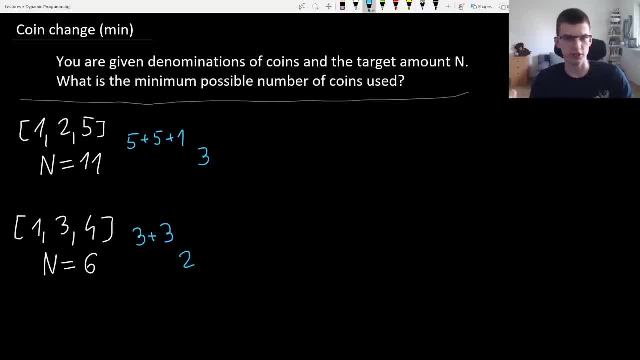 which gives me the answer 2.. Again, you can think about a greedy approach, because this is optimization problem, and if you every time take the biggest possible coin for n equal to 6, maybe you would want to take 4 first and then the remaining value is 2, you need to make 1 plus 1, this is not. 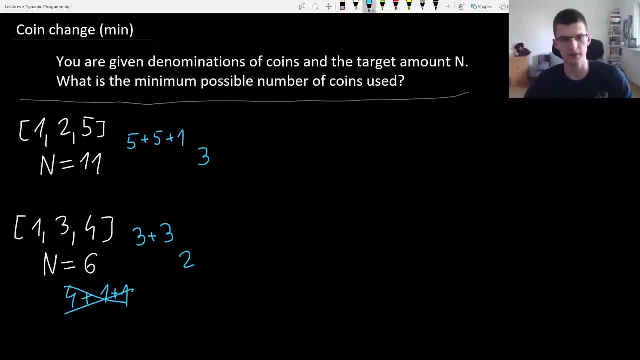 optimal. This means the greedy doesn't work here And the code will be very similar in the solution. The solution will be very similar to the previous one. it's just that dp of i instead of being the number of ways to get this sum, it is the minimum possible number of coins. 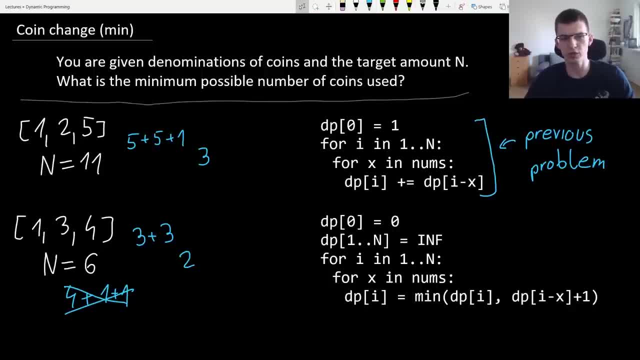 Let's see comparison of two implementations. I took the first code and slightly modified it. The initialization is different. I can't leave everything to be 0, because then I will think that dp of n is 0, that 0 coins are enough to get the sum of n. 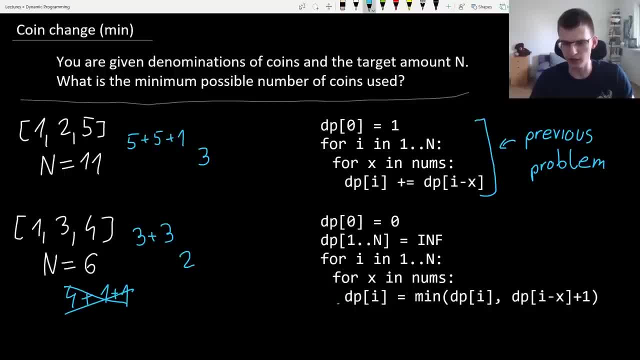 But if we know To compute dp of i, I iterate over the last coin and I find the minimum over dp of i minus that last coin. i minus x is the sum so far before that last coin, plus 1, because I'm using one more coin. 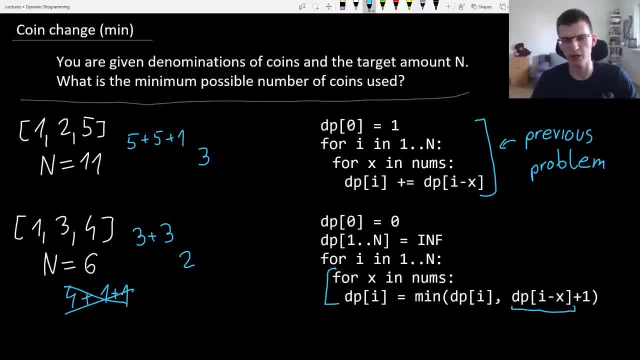 I could also put that plus 1 outside the bracket, but I mean I could find the minimum over dp of i minus x and only then add 1.. But it doesn't matter. In this code and the previous one, what you should be careful for is, of course, out-of-boundaries. 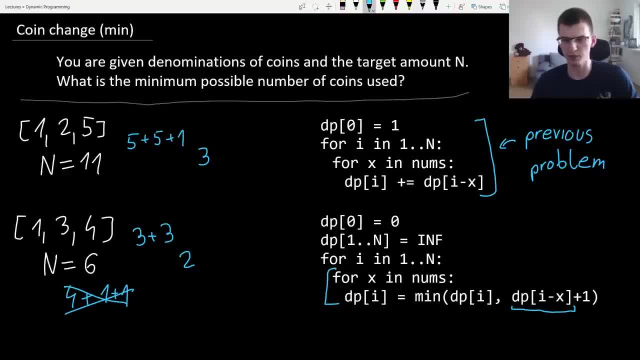 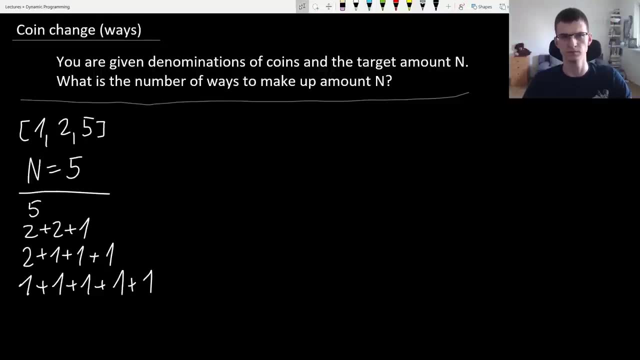 error. This is pseudocode, but in actual implementation you need to check whether i minus x isn't negative Plus. here we initialize all the values to infinity and the sum equal to 0 you can get with 0 coins. This problem is certainly the hardest in this lecture. 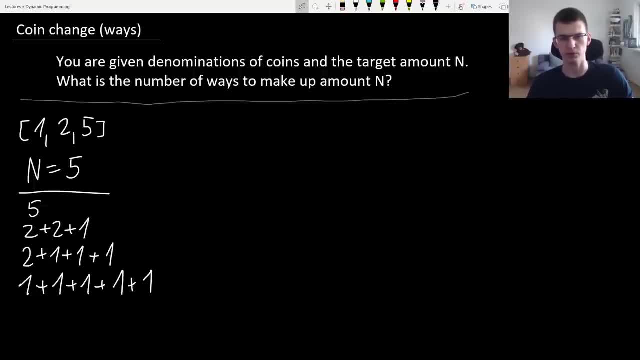 It's again coin-triple. The number of coins in the set of numbers doesn't change, but this time we're counting the number of ways We are given denominations and the target amount n. what is the number of ways to make up that amount? 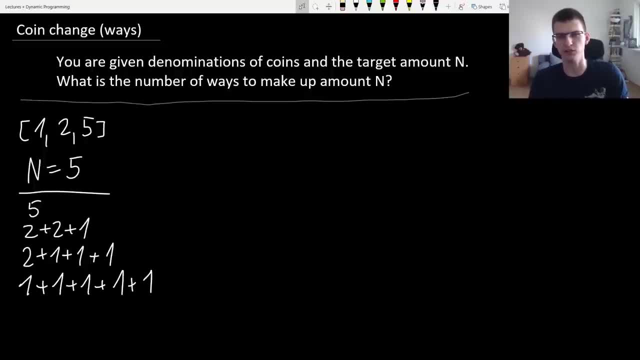 This time, though, we say the order of numbers doesn't matter. What matters is multi-set of coins. If you're in a shop and you want to choose bunch of coins to pay exactly n, then the order of them doesn't matter. You don't give those coins one by one. 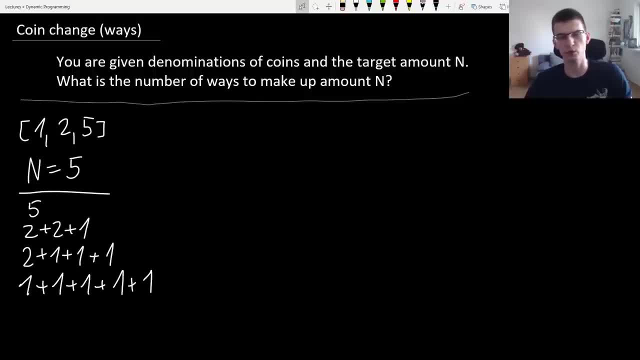 It becomes one place where one and two are equal. At the end of our lecture we also discussed two problems ago from combination sum, where we're? we were writing n, as the sum of numbers and is 2 is equal to 1.. 1, 1, 2 was counted separately from 1, 2, 1.. 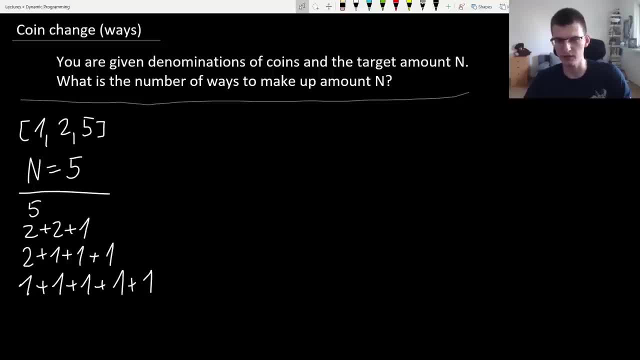 Here the target value is 5 and coins are 1,, 2, 5.. There are four ways that I wrote on the left. If we would count every order separately, Then instead of just 2 to 1.. then also 2, 1, 2, 1, 2, 2, and similar thing for 2, 1, 1, 1.. There would be four ways. 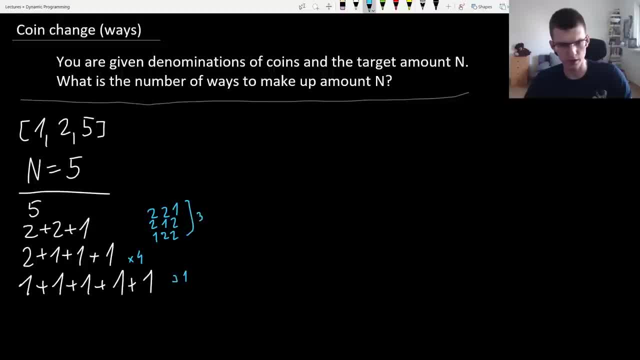 Here I have 3,, 4,, 1 and 1. The total would be 9, but this is a different problem. The order doesn't matter and the answer is 4.. If we just applied the same dynamic programming that for some already chosen elements remembers the sum here: sum. 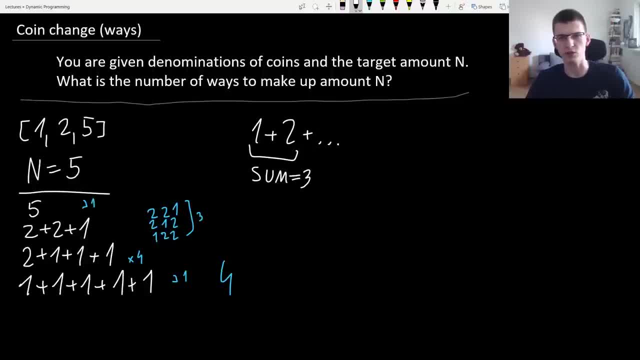 equal to 3, we would get the issue of double counting or over counting. We would separately count way with 2, 2, 1, 2, 1, 2 and 1, 2, 2, because all of them give us the 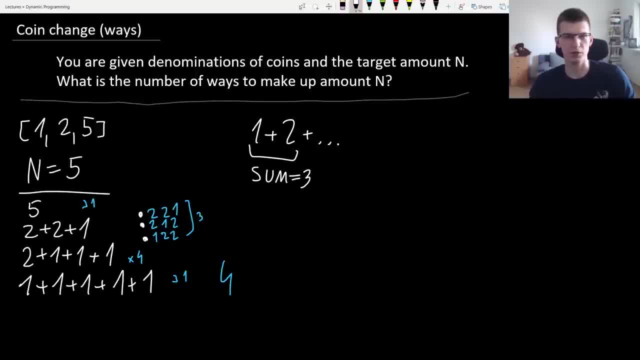 sum n in position dp of n. We need to change something, and now not only we need to change something, and now not only the sum matters. we cannot say dp of i is the number of ways to get sum i, and that's it, because we don't want to double count any state, any solution And 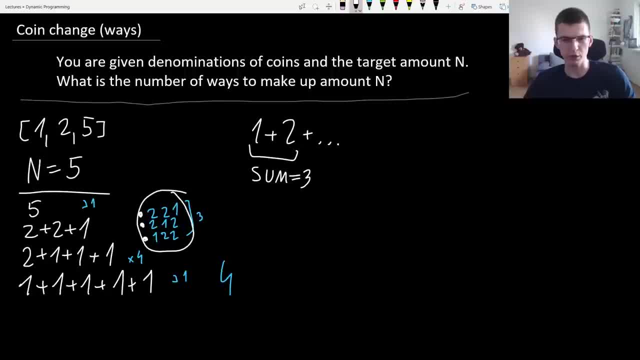 not to count those three separately. I will say that I want to only allow one of them. What makes sense is to count the lexicographically sorted way. This is a unique representation of all of those. I want to not allow those two. Then, in our already chosen 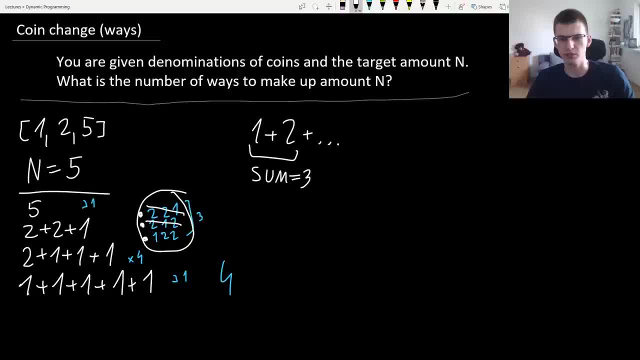 elements. not only the sum matters, but also the last element, And the next element cannot be smaller than that. This time we'll say that dp of s sum and k let's, instead of k, use last. this is the number of ways to get the sum of s, where this is the last used coin. 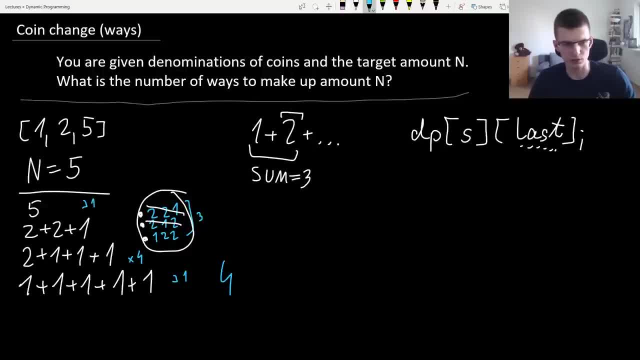 If we number coins from 0 to k minus 1, where k is the number of them, then the memory complexity of our dp this time is of n times k. s is up to n and last is up to k minus 1 and every state with sum sum. 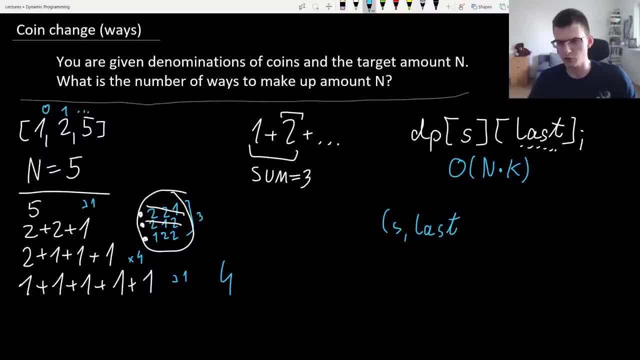 sum, sum and last, we should iterate over the last coin taken. maybe We'll think about that in a moment, but the trivial approach here would lead to time, complexity and k square if you want to iterate over the last coin, but it won't. 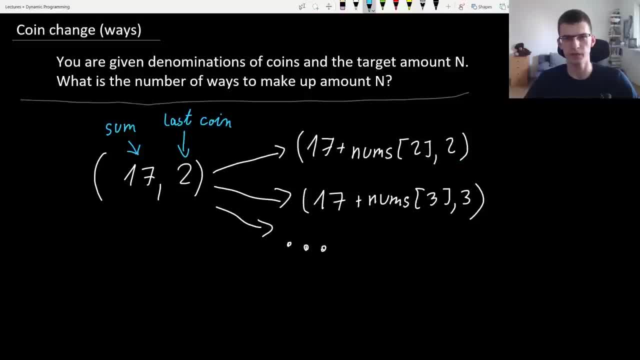 be necessary and we will get n times k. If the state is sum so far and the last coin, then let's say last coin had index 2, the next coin can be coin 2, coin 3,, 4 and so on, If we choose the next. 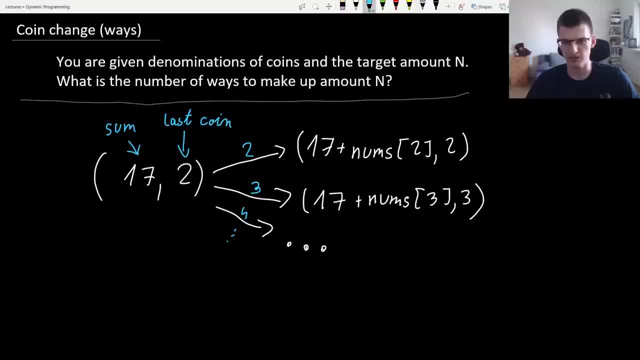 coin to be 2 again, then the new sum is 17 plus the value of that second coin. in the array nums, the last coin is still 2, then 3, and so on. From each of n times, k states, we consider k transitions. This is why the complexity is n? k square. We 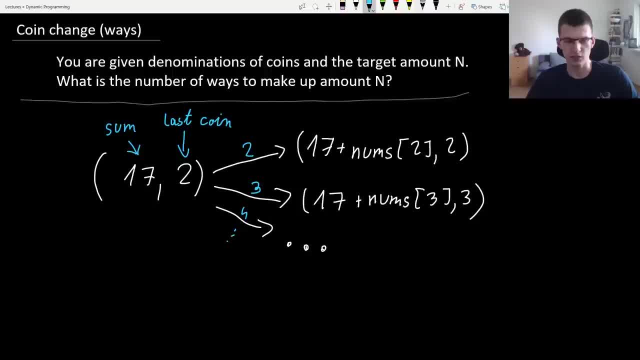 also know that n times k is the sum over dp of n, the target value, and the last coin can be just anything, the sum over all those question marks. How to make the time complexity n times k, though? It's very simple. it's enough to say that from. 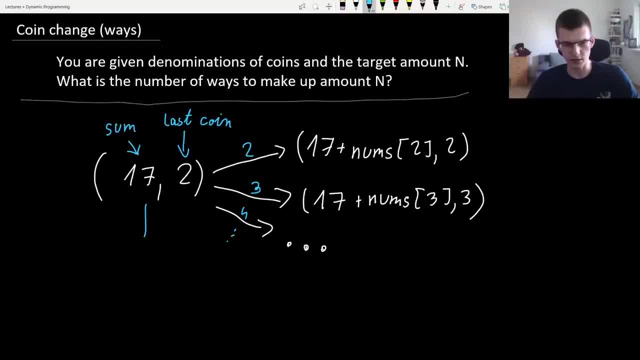 state 17 and 2, you can get to state 17 and 3.. You can imagine that last coin is 3 and from that state you will consider cases where the next coin to take is 3 or 4 or whatever else. Then you remove all those. 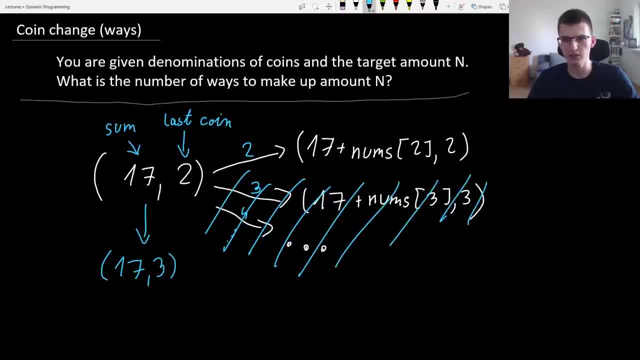 transitions and you have only 2.. Actually this changes the definition of last coin a little bit. This is not the last coin but kind of the limit for the coins that you used or you can use. So if we don't choose coin 3 or lose K3, if we use the last coin to take, we are 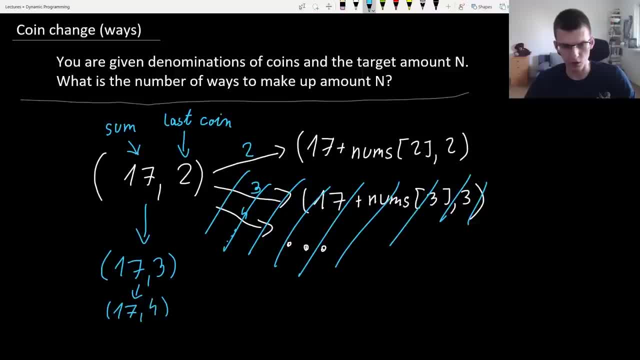 already gave 2 values. Anyways, if you used coins 0,1,1 and 4, you can say that the last coin is 4, if you aren't going to take smaller coins. If you write it this way, and from 17,3 we can get to either 17,4 or to. 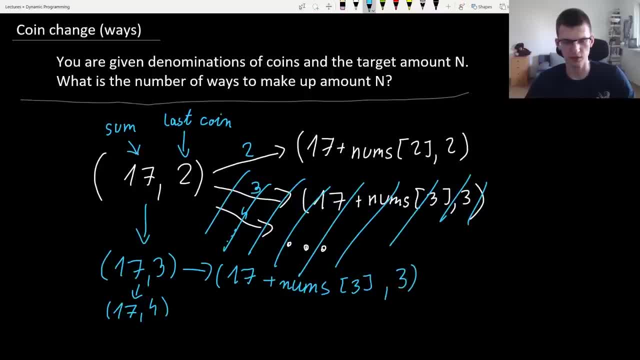 now comma 3, which is the last coin, then we are fine. every possibility, like taking, for example, coins 0 then 1, then 1, 2, after that 4, 4 and so on, every possibility like that will be counted and what is important is it will be. 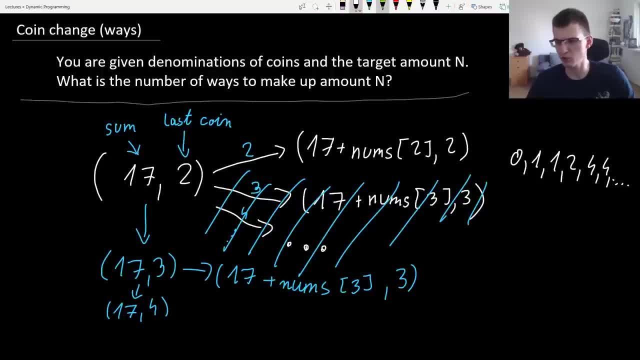 counted exactly once. when, after taking 0, 1, 1, 2, we are in this state, then we don't need to iterate over all those coins that we take next. it's enough to go to state that thinks the last coin so far was free, because we don't want any more. 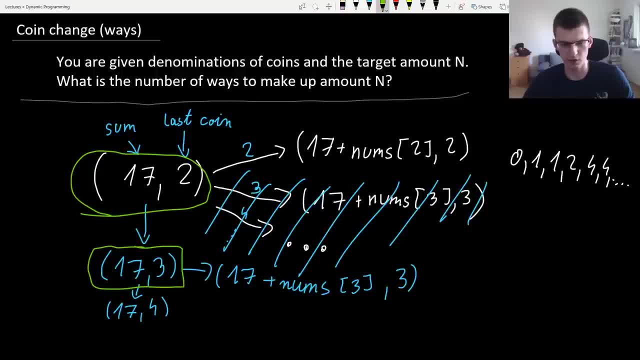 coins of index 2, then we'll go to 17, 4, and from that we'll get to that 17 plus nums of 4, comma 4, which represents taking coin 4, and this doesn't double count anything, because in that graph of transitions there is only one path that corresponds to this multi set. 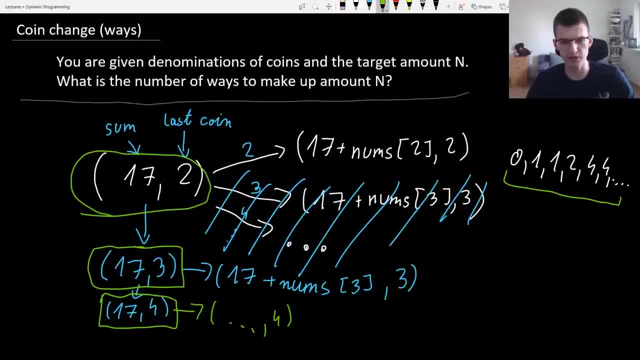 of coins. it must go like this: if from 17- 2, we go with the other transition to this state, that would represent taking another 2 when we have already 0, 1, 1 and 2, then either the next coin is 2, in that case we go to that state where we still. 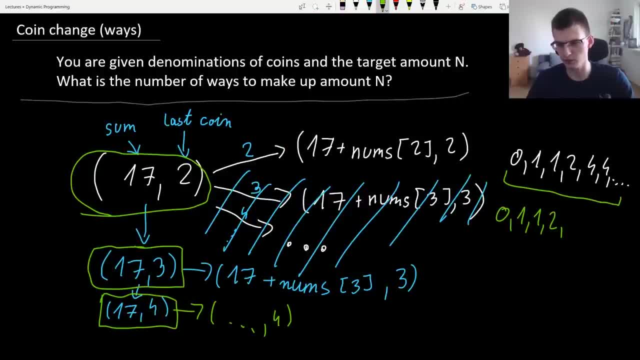 can take 2s. otherwise, if it's not a 2, it's if it's 3 plus. then we go to the next state below 17 and 3 in the graph of transitions. there should be exactly one path, and then there is no over counting. one more thing for this. 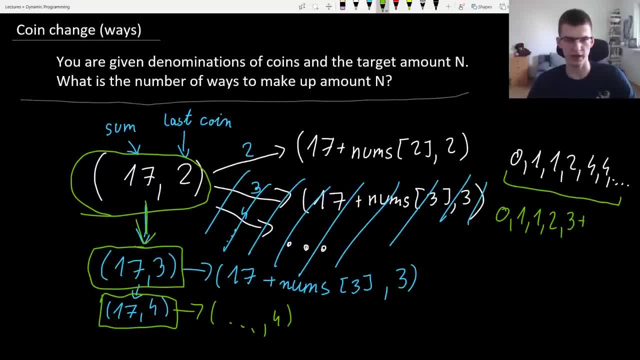 problem is that you can get memory O of n, like for those, instead of having dimension k, you go coin after coin and for every next coin, from 0 to K minus 1, you update the DP of i. then DP of i would be the number of ways to get this. 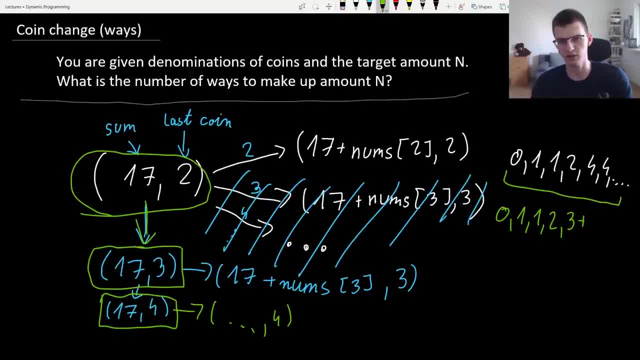 sum i with coins. considered so far, actually this is very similar to knapsack and we'll talk about it in one of future lectures. but yeah, memory can also often be optimized by one dimension. What we described so far has both time and memory. complexity of n times k. 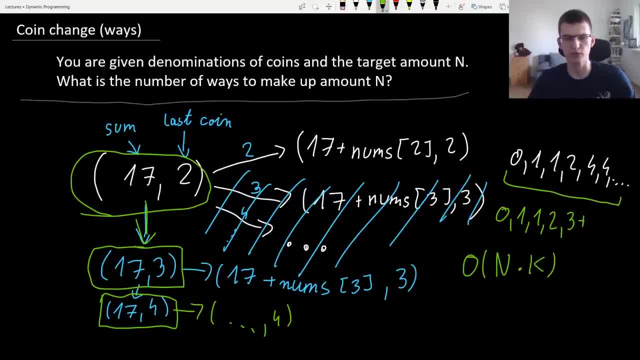 The number of states is n times k and we have just two transitions. You might notice that we actually did that: forward DP or push DP. It's also possible with pull or standard. take from previous values DP where DP of i last is computed from previous states. then 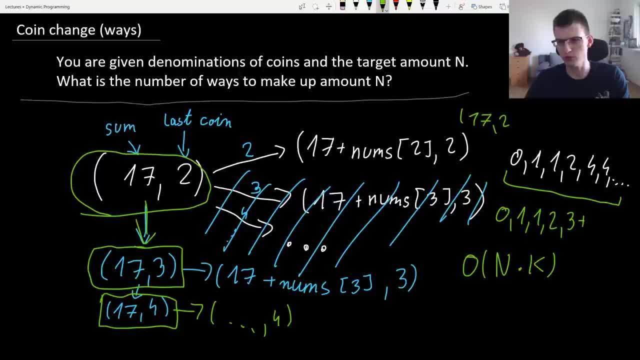 DP to that 17, 2. you need to go from 17 minus nums of 2, nums of 2 comma 2, or from 17, 1. It's the same thing. There are just two ways to implement that. If you want, try this. 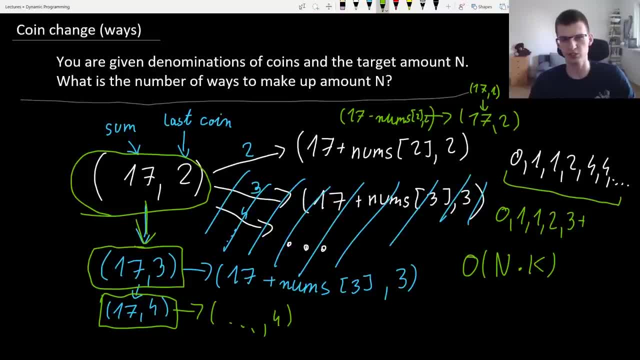 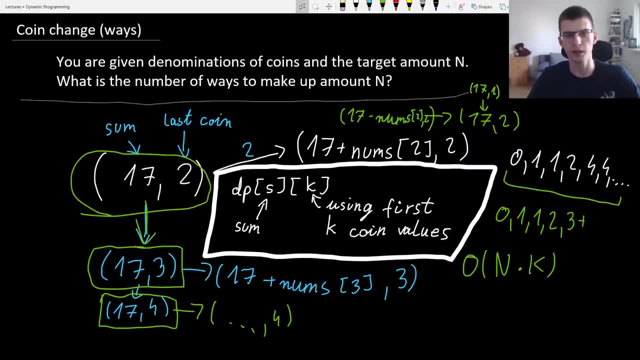 problem or one of previous two. there will be links in the description or in the pinned comment- the first comment below the video- So you can try to implement this yourself. I mentioned already that the second value of the state that last coined isn't really the last coin. 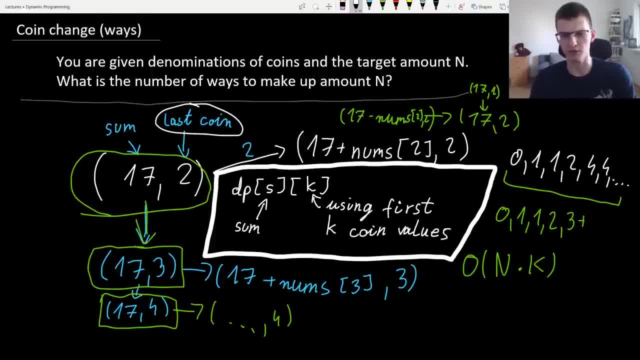 It's our limit and there is a concise way to now define the state of DP. DP of s, k is the number of ways to get the sum of coins already used equal to s, where we used only first k denominations. From that array nums, we were allowed to only use first k values and 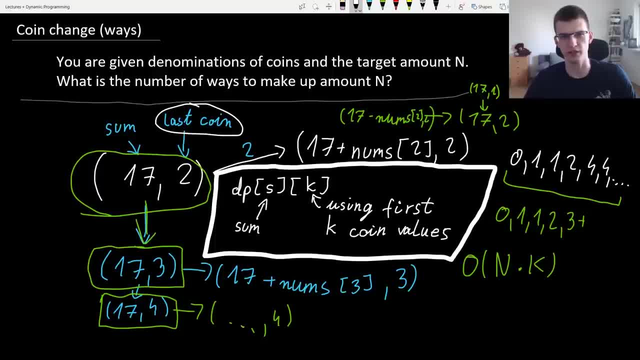 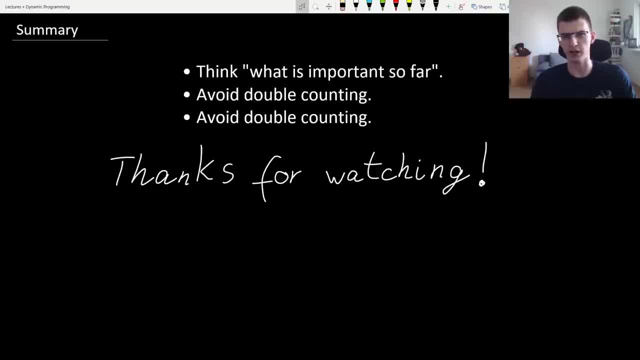 then there are indeed just two transitions from every state From this lecture. you should remember that in dynamic programming problems you must think what is important so far, after we made some decisions, after we already chose some numbers or in graphs, after we got to this vertex In